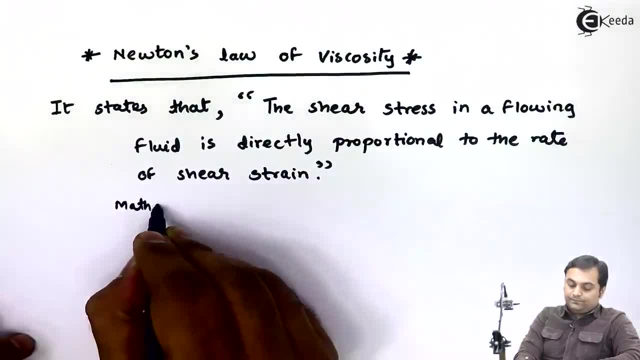 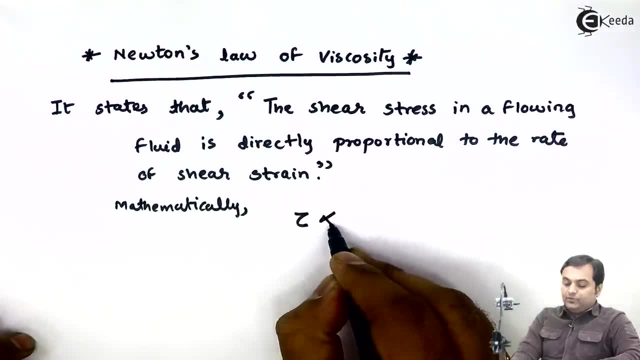 So therefore, mathematically, shear stress is denoted by tau and it is directly proportional to the rate of shear strain, which is nothing but change in velocity, du upon the change in distance, which is du. Once I replace the coefficient of proportionality here, I have mu into du by dy. 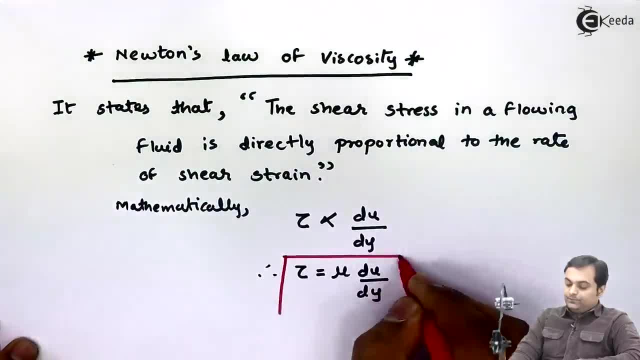 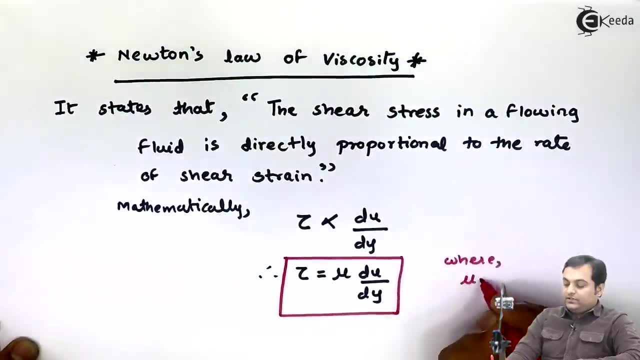 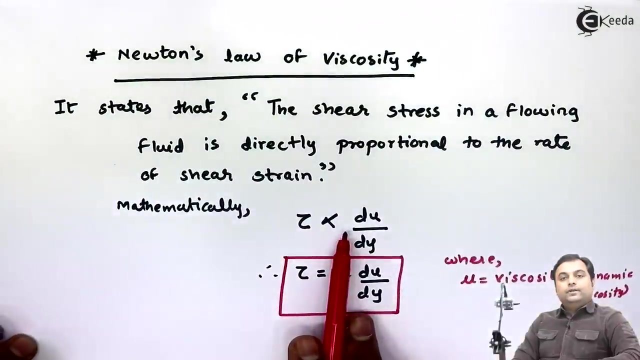 So in other words here I can say that where mu is called as viscosity or it is just called as dynamic viscosity, So shear stress is directly proportional to the rate of shear strain. This term du by dy, it is called as rate of shear strain. 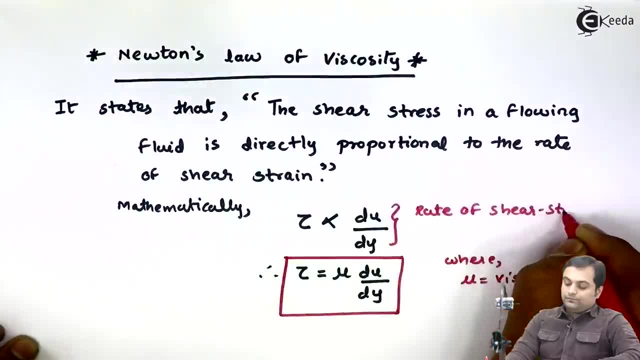 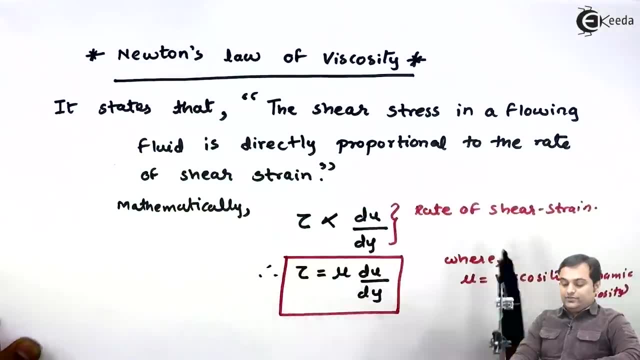 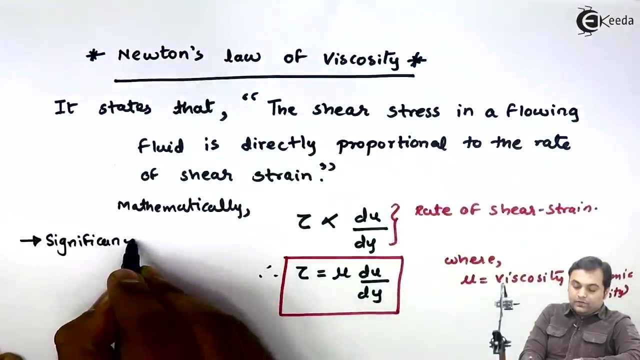 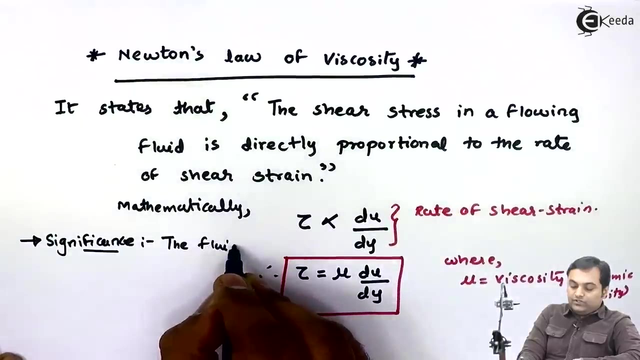 And when shear stress is directly proportional to the rate of shear strain. that is called as Newton's law of viscosity, And its significance is directly proportional to the rate of shear strain. Now talking about the demand alpha in the fluid circuit. Now talking about the demand alpha in the fluid circuit. 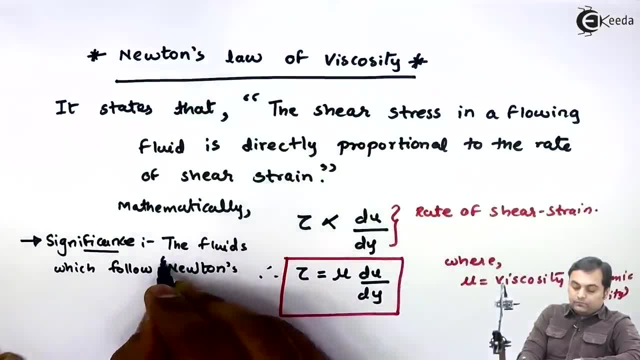 The top worst grupo is that the fluids which follow Newton's law of viscosity are called Newton's law of viscosity. The wave of velocity increases. when a wave of velocity increases, The period that a wave of wave exceeds is known as Newton's law of velocity. 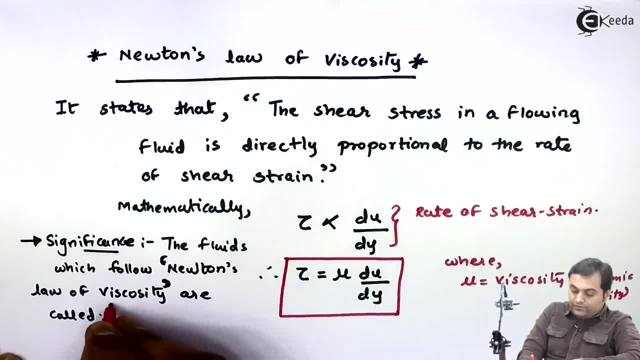 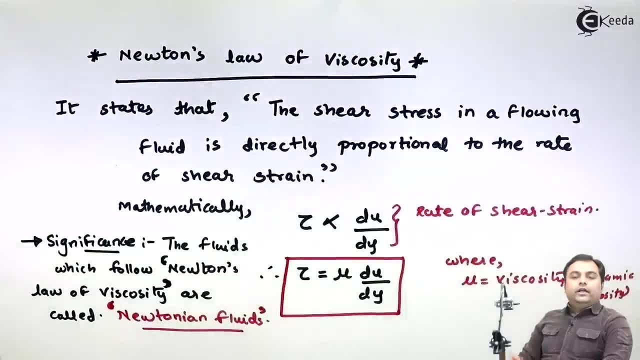 Newtonian fluid. so here is the significance: that if a fluid it follows Newton's law, that is, if in a flowing fluid the shear stress is directly proportional to the shear strain, then we can say that the fluid is following Newton's law, and when it follows Newton's law it is called as Newtonian. 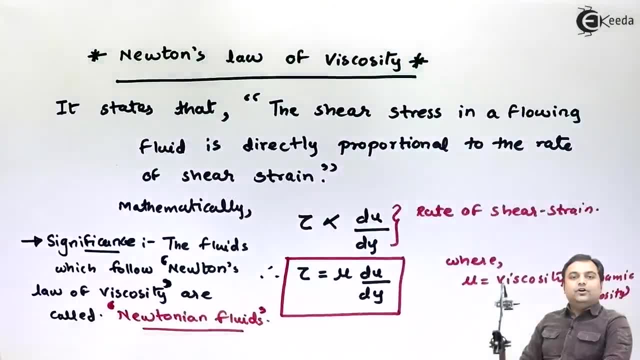 fluid. so here we have seen in this video what is the meaning of Newton's law of viscosity.